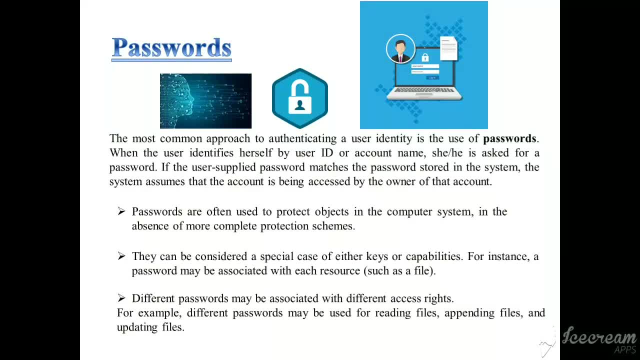 The most common approach to authenticating a user identity is the use of passwords. When the user identifies herself by user id or account name, she or he is asked for a password If the user's supplied password matches the password stored in the system. the system. 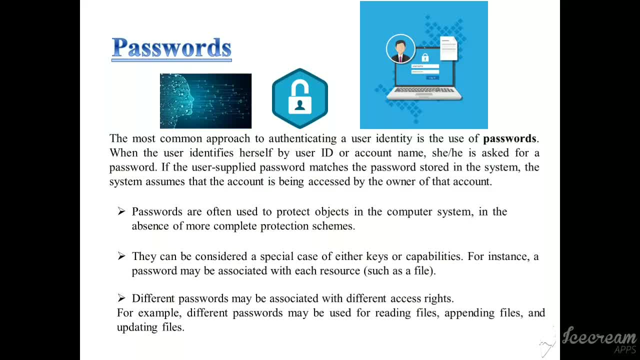 assumes that the account is being accessed by the owner of that account. So nowadays, by starting stage for securing our systems and our personal electronic devices, we are commonly using passwords. So passwords is very security. it gives a security so no one can access our personal. 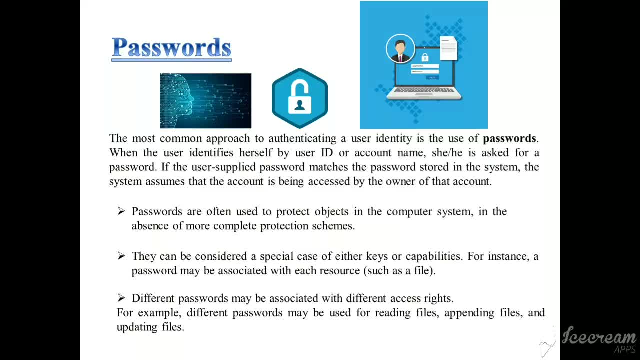 data or systems or any other devices without password. So owner can only access the device by using username and password. Passwords are often used to protect objects in the computer system in the absence of more complete protection schemes. So passwords are being used in computer devices also to protect data and files. They can be 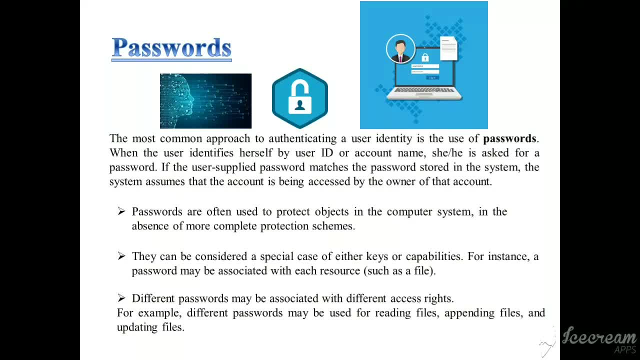 considered a special case of either keys or capabilities. For instance, a password may be associated with each resource, such as a file, So we can keep the password for each single file also. So it is easy to keep the password and access it. 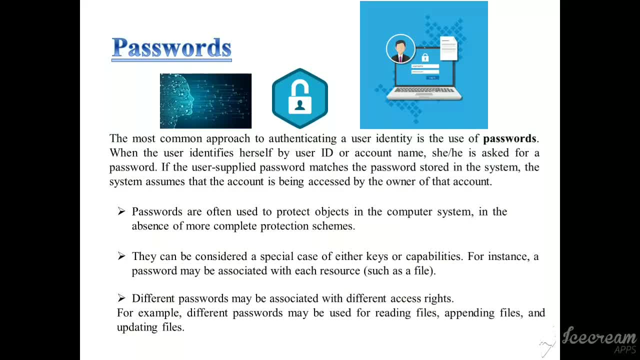 It gives a security. Without password, no one can access our data or files anonymously. Different passwords may be associated with different access rates, So all passwords are not same rates. It has different access rates. It is read-write reading files appending. 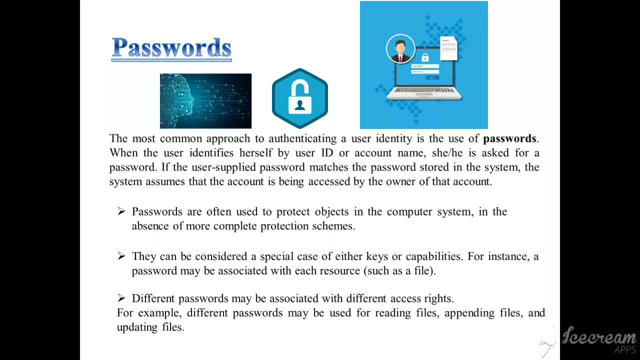 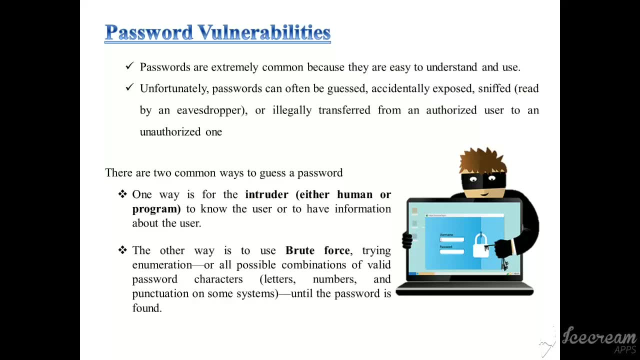 files and updating. So we have different types of passwords for each process. So next let's talk about passwords- Passwords. So next we discuss what are the disadvantages or risks of passwords. Passwords are extremely common because they are easy to understand and use. So it's easy to understand and use. 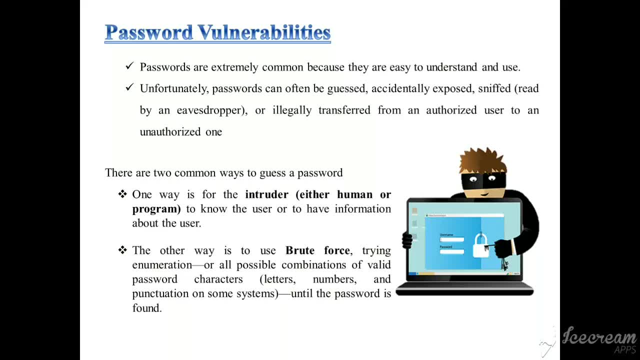 So passwords are used everywhere. Unfortunately, passwords can often be glissed, accidentally exposed or snipped read by a dropper, or illegally transferred from an authorized user to an unauthorized one, So passwords can be easily glissed by anyone. So like we are using our date of birth or 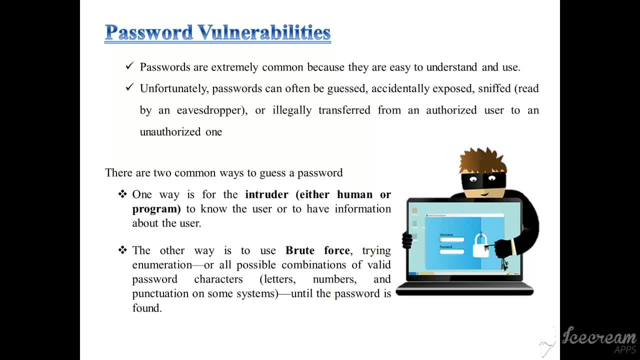 name. any other name or a persons name So easily can be glissed and accidentally exposed In case if you want to access anything in other system, means in another system. we are given passwords so it can be exposed Razor. So there are two common ways to guess a password. one way is Intruder- either a human or program. 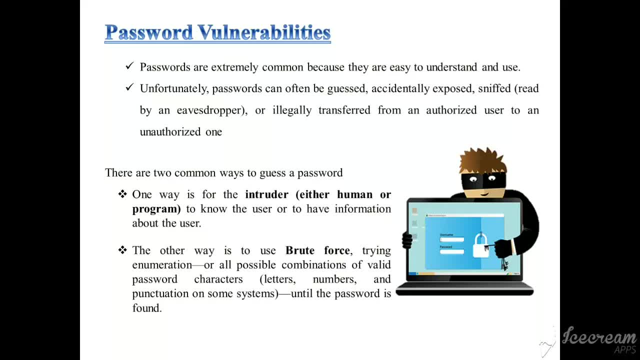 to know the user, to have information about the user, So human can guess or see the passwords anonymously without knowing our knowledge. so it is one way. The other way is brute force technique, trying enumeration or all possible combinations of valid password characters, letters, numbers and functions on some system until the password. 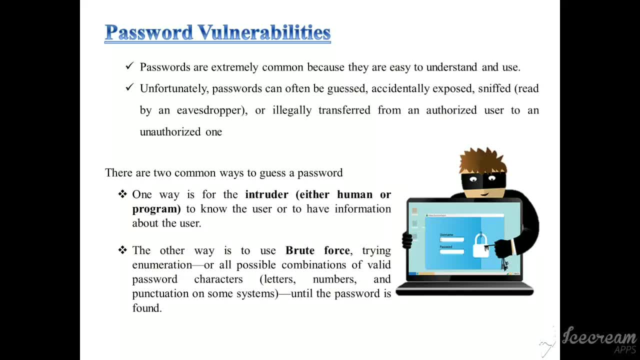 is found. So brute force technique is a very powerful technique to hack the password. so it is. it matches the combinations passwords from starting, so within 5 minutes it can access 10,000,. it can match 10,000 possible passwords. correct passwords. 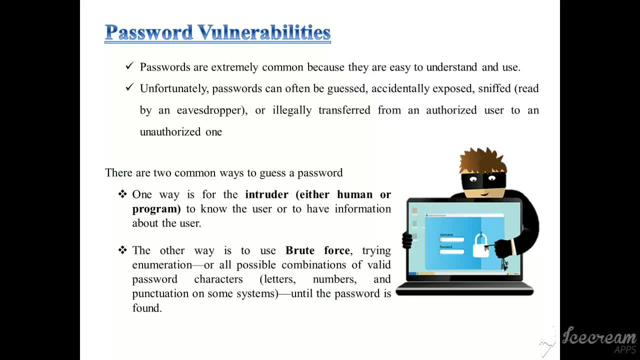 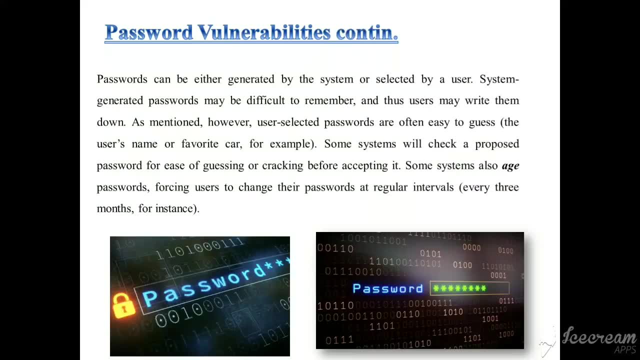 Ok. So it is very powerful technique, one of the best hacking technique using brute force. So passwords can be either generated by the system or selected by a user. system generated passwords may be difficult to remember and thus users may write them down. So passwords are generally generated by two ways. system generated passwords may be difficult. 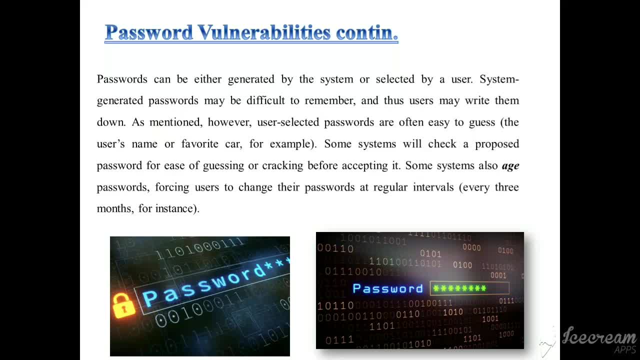 to remember and thus users may write them down, so it is difficult to remember. So, as mentioned above, user selected passwords are often easy to guess. So if you, we want to select or we select the password we are selecting, choosing easy. 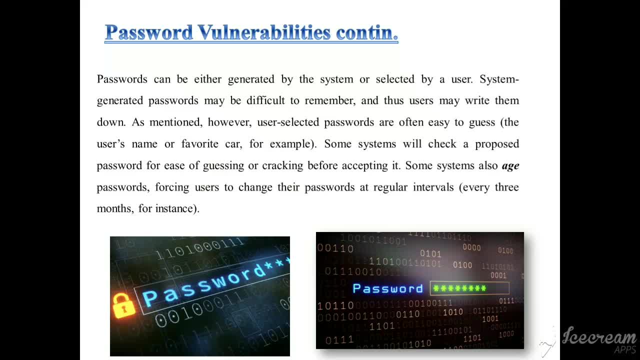 passwords, so it is easy to remember and guess. Some system will check a proposed password for ease of guessing or cracking before accepting it. Some systems are also easy to remember and guess. Some systems are also easy to remember and guess, So EasePassword, forcing user to change their password regularly to work every three months. 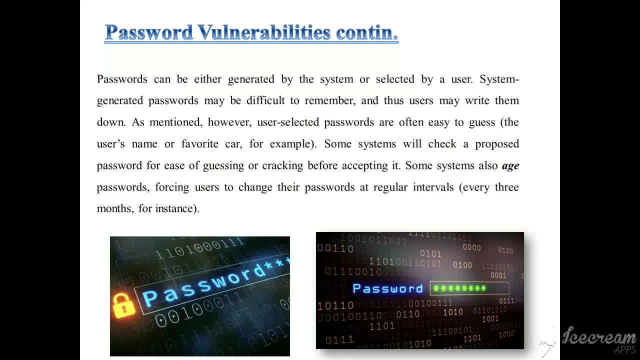 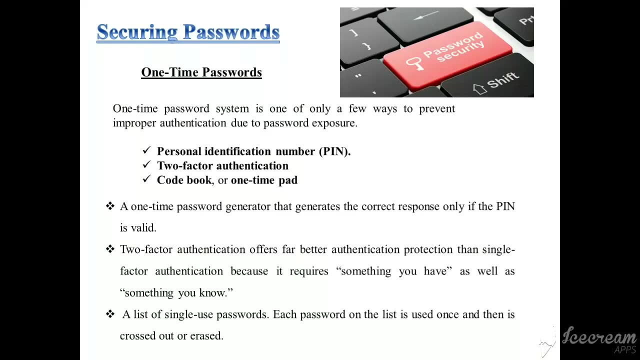 for instance, Some systems are automatically- they are showing error or interrupt- to change the password to secure more. So next, securing passwords. so we have different techniques to secure passwords. So we learn one by one One time password, called as OTP. one-time password system is one of the only a few ways to prevent. 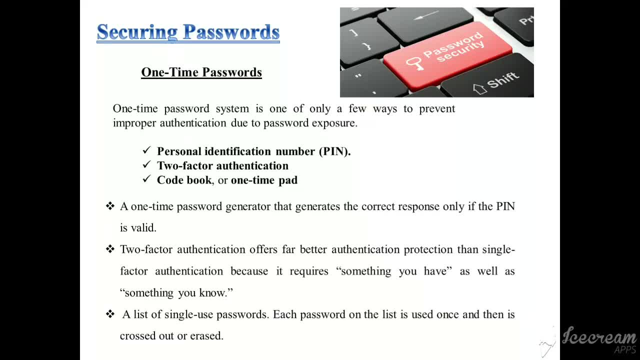 improper authentication due to password exposure. so it contains personal identification number, pin, two-factor authentication codebook or one-time pad, the one-time password generator, that generates the correct response only if the pin is valid. so if the pin is valid then it will login, otherwise it will. 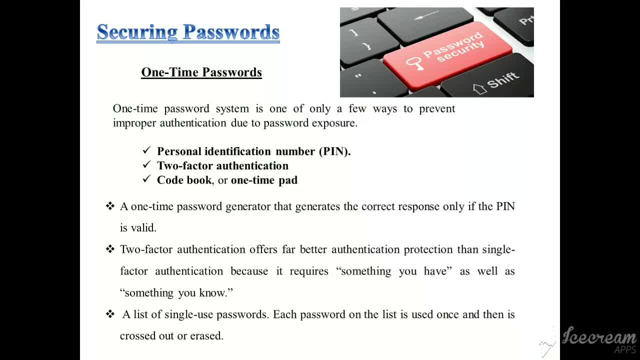 block the user. two-factor authentication offers far better authentication protection than single factor authentication because it requires something you have as well as something you know. so two-factor authentication means if you want to log in to any systems, the pin or password will messaging to our mobile number if we registered mobile, so using that password. 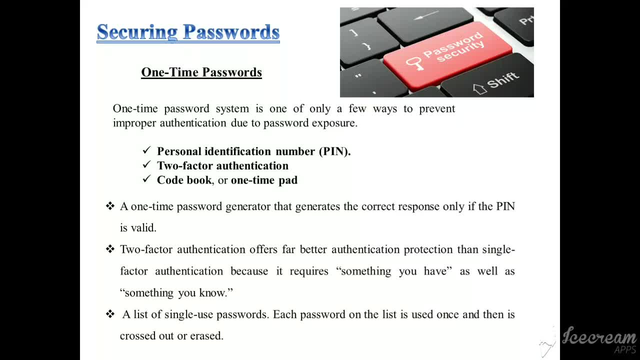 we can log in. so it use user setting password and OTP, both a list of single use password. each password on the list is used once and then is crossed out or erased. if you once we use one-time password, it will be erased, so next time it will generate a new one. 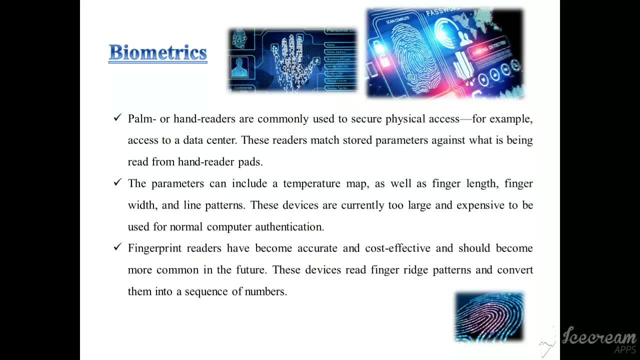 so next technique is biometrics, so it is very powerful. security features in user authentication, clamor and readers are commonly used to secure physical access, for example access to a datacenter. these readers may store parameters against what is being read from the and reader pads, so the parameters can include a temperature map as well as finger length.